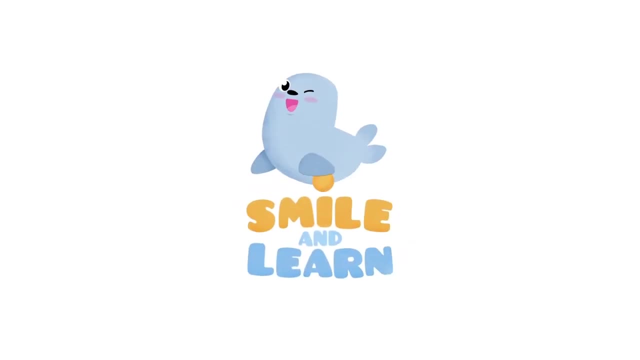 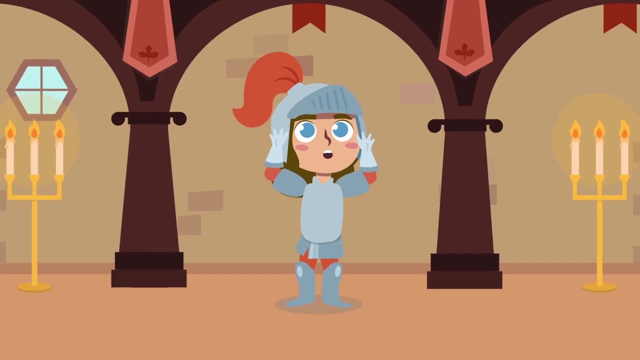 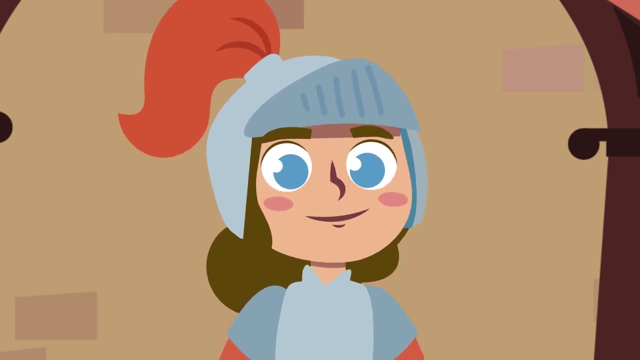 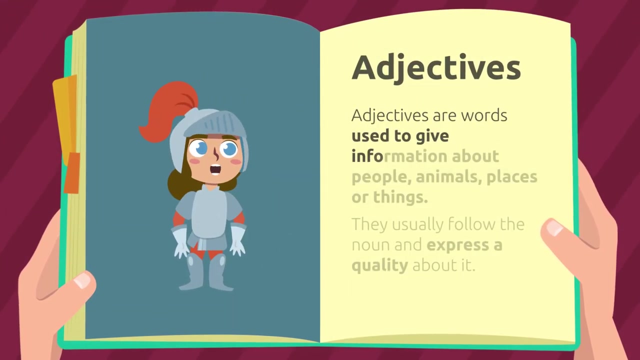 How are my word lover friends? Today we'll continue learning more adjectives. What do you say? Do you remember what they are? If not, I'll remind you. Adjectives are words used to give information about people, animals, places or things. 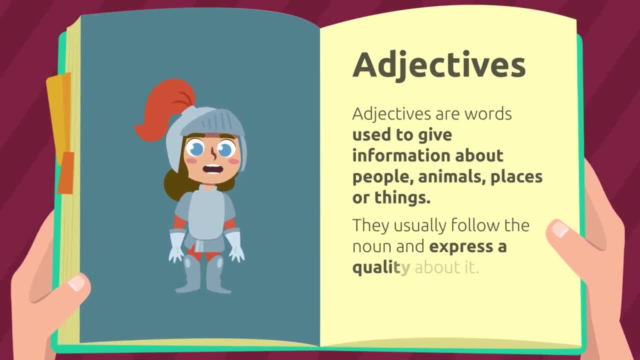 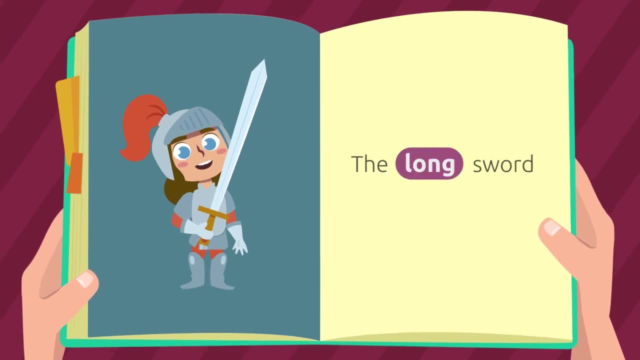 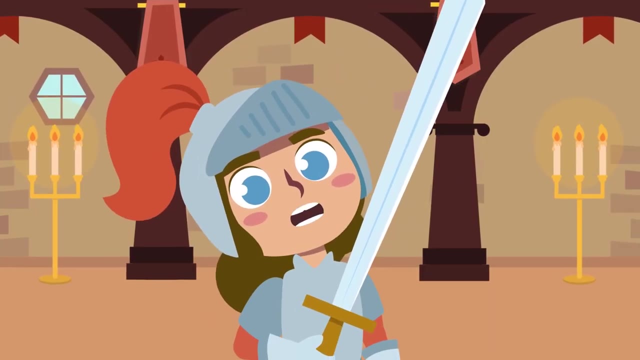 They usually follow the noun and express a quality about it, For example, in the sentence the long sword- Long would be the adjective because it tells us what the sword is like. In this video, we're going to learn about some adjectives that describe qualities about different. 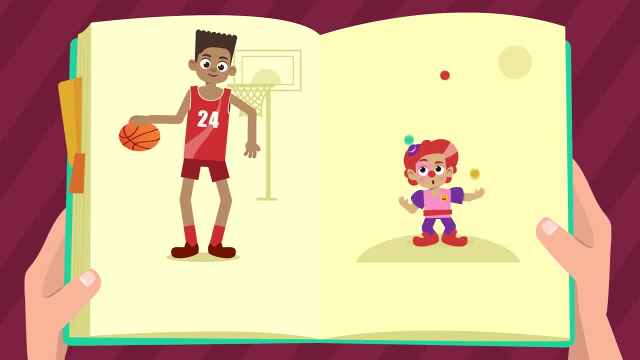 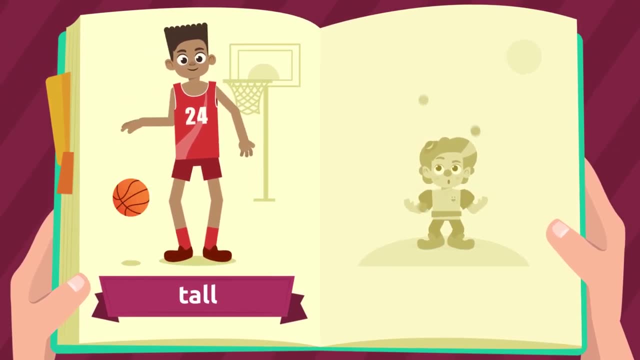 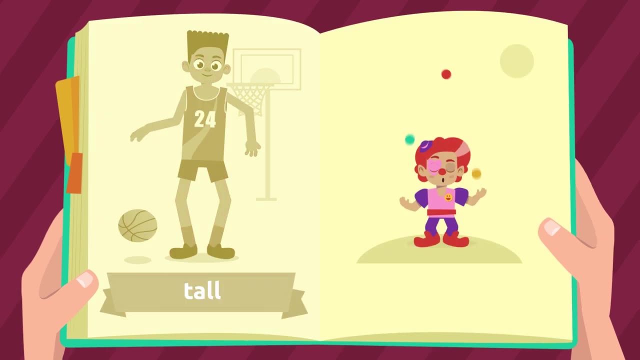 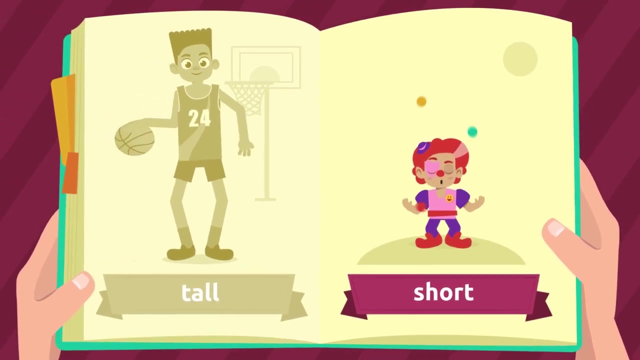 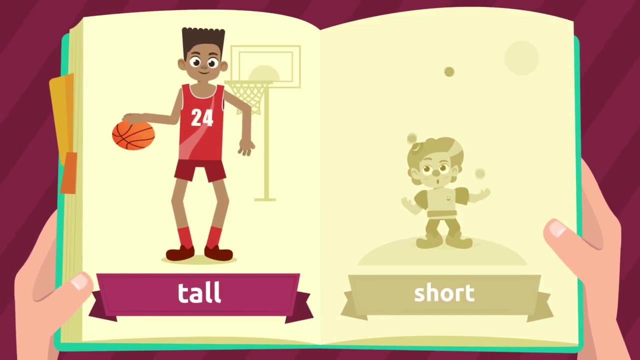 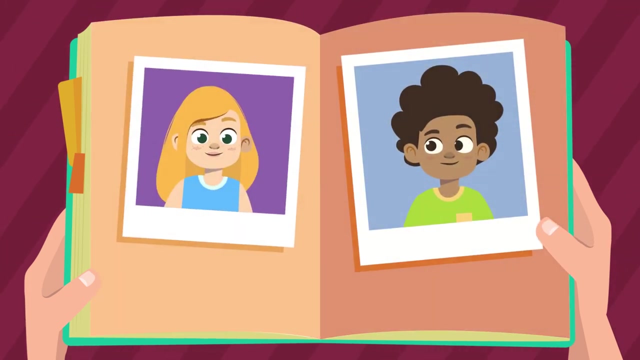 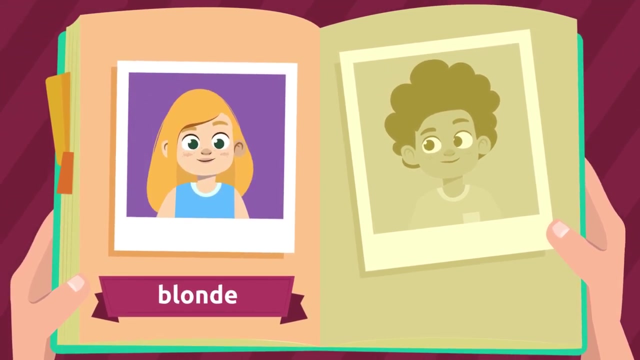 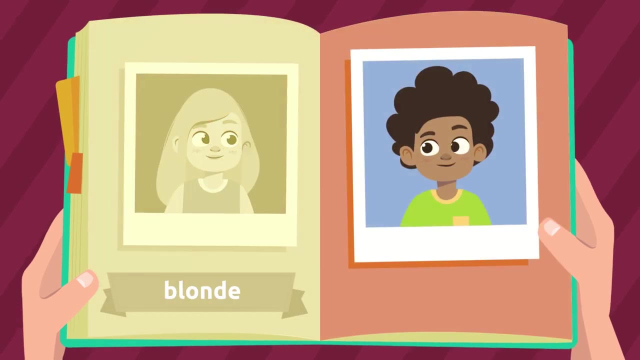 people. Here we go. This basketball player is tall, Tall, Repeat after me Tall, But this clown is short, Short, Repeat after me Short, Tall, Short. Paula has blonde hair- Blonde- Repeat after me Blonde. And Miguel has brown hair- Brown- 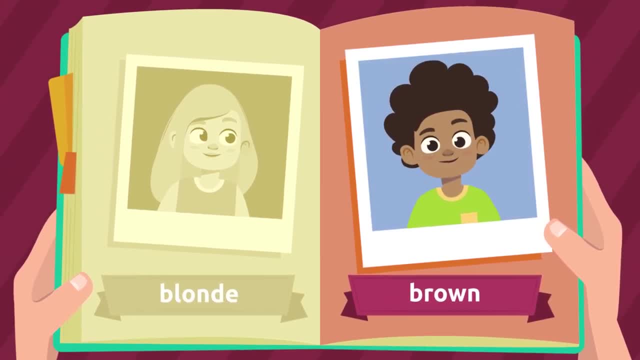 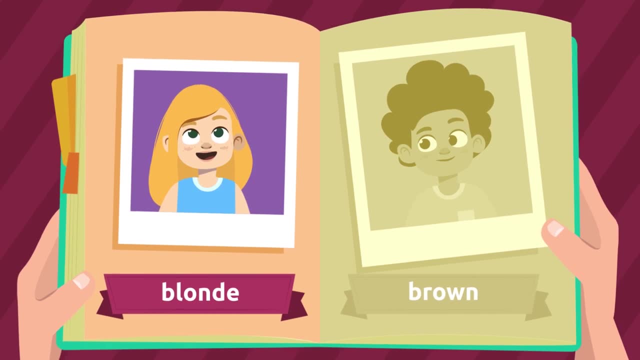 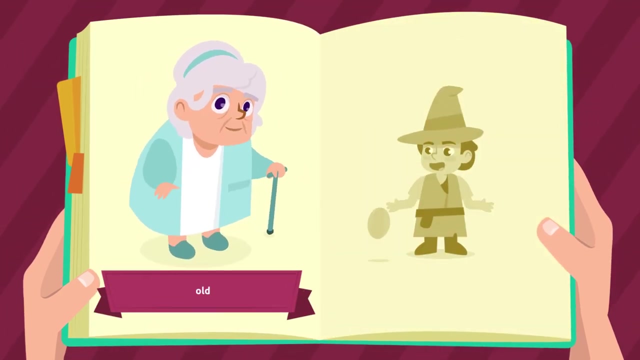 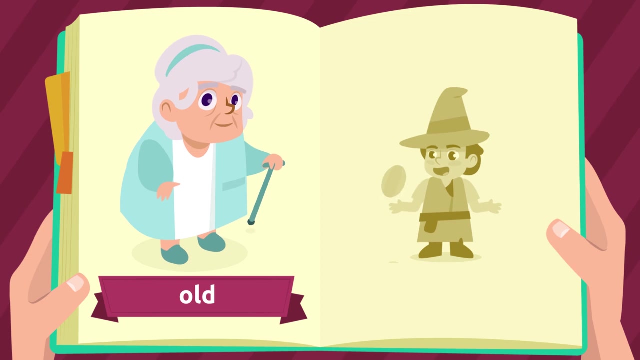 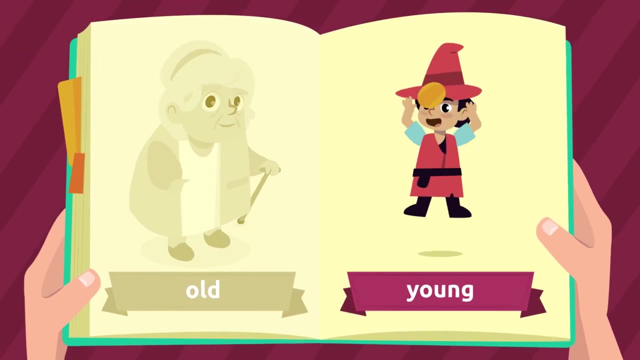 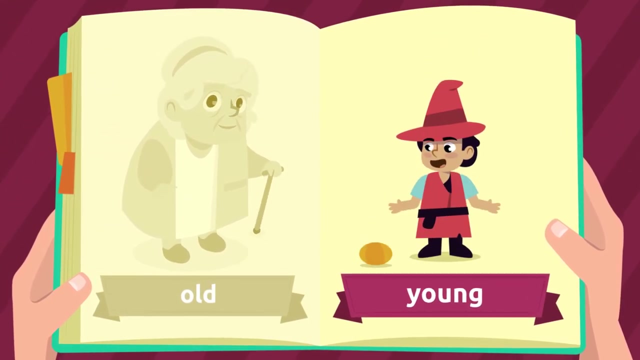 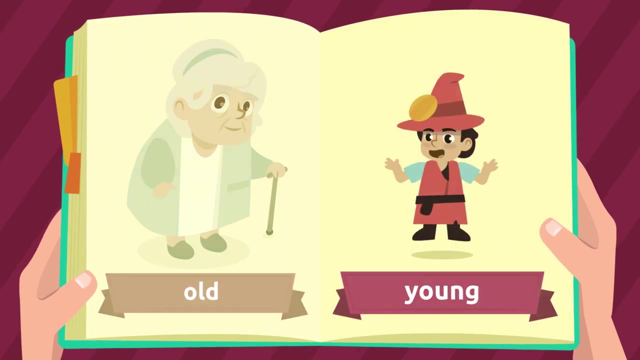 Repeat after me: Brown Cya later goin' on a date. We're eating lunch at Franco's And they're competit Ram executed there. Look out, We're going on a date. This boy is young, young. Repeat after me: young, old, young. 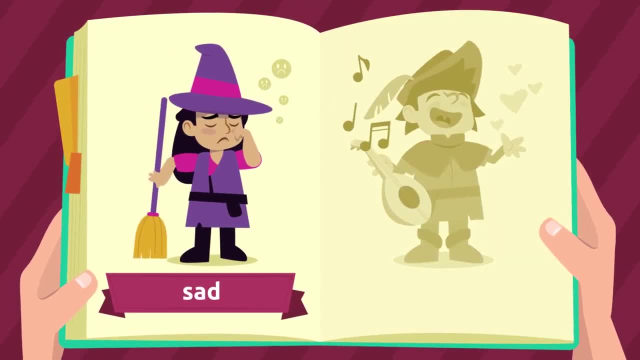 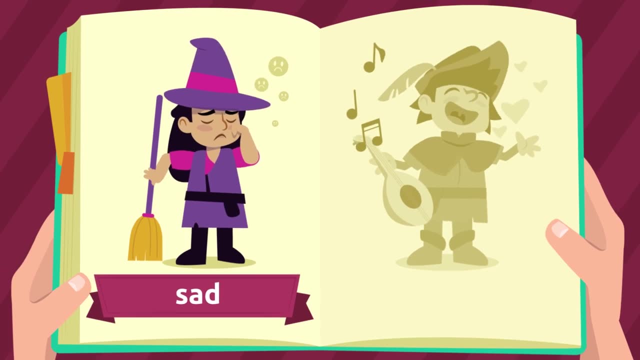 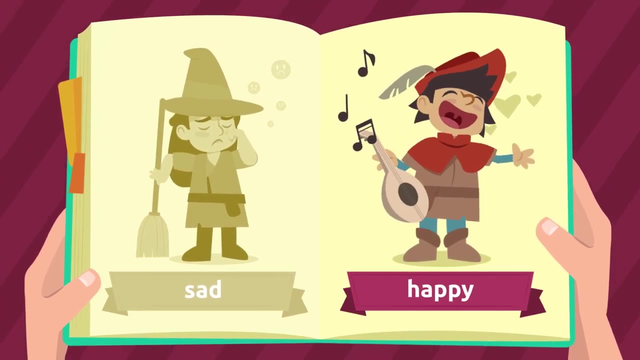 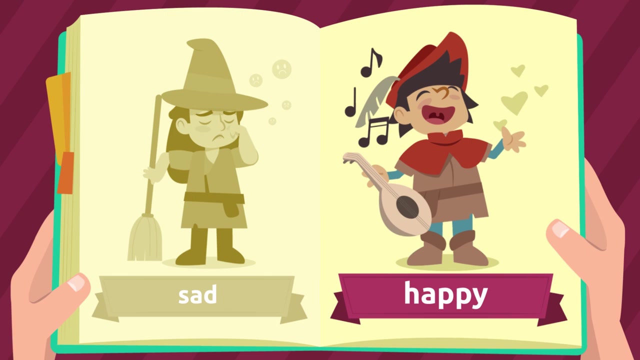 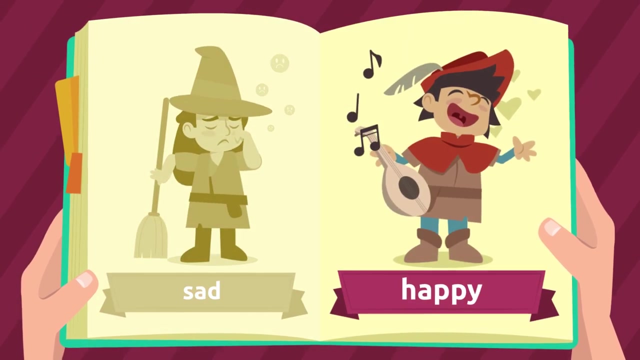 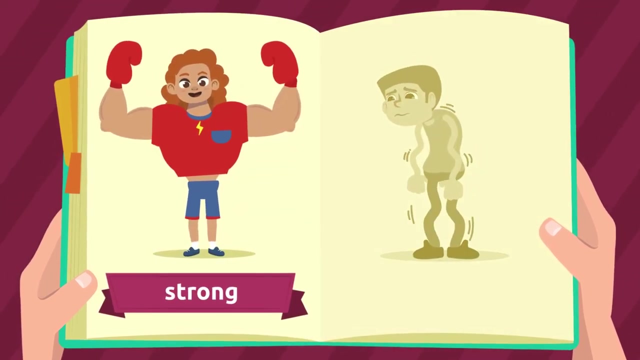 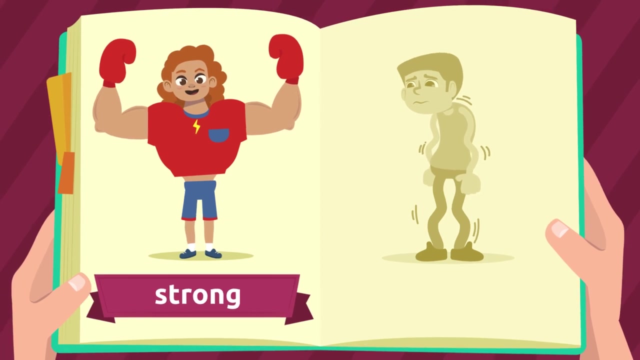 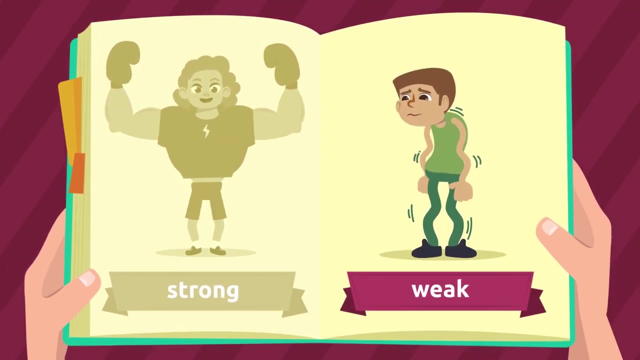 This witch is sad, sad, Repeat after me sad. But this musician is happy, happy. Repeat after me: happy, sad, happy. This boxer is strong, strong- Repeat after me: strong, But this boy is weak, weak. 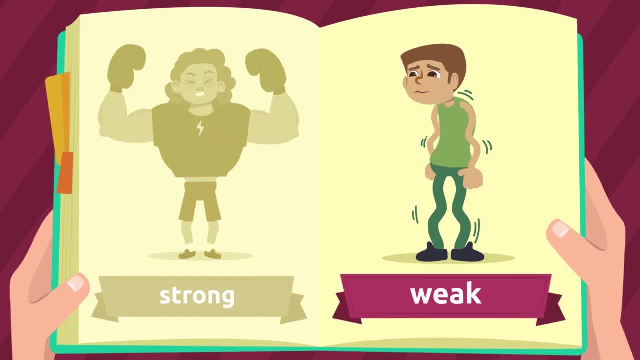 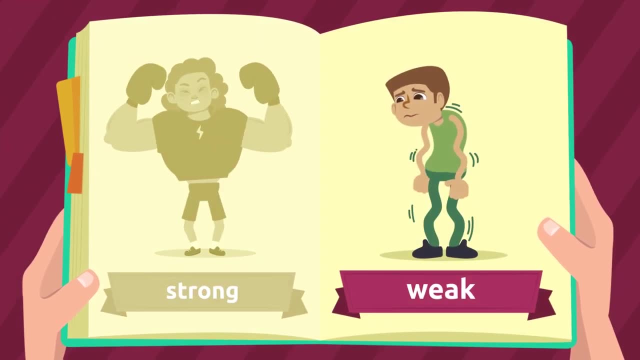 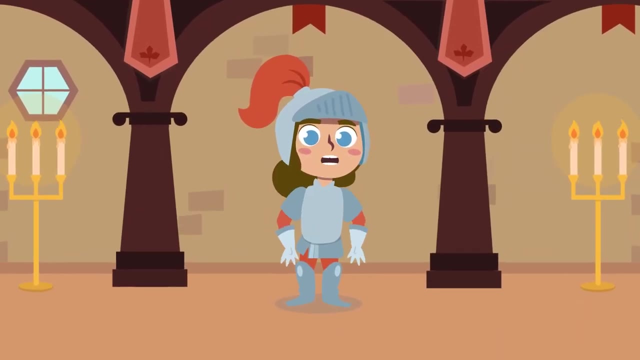 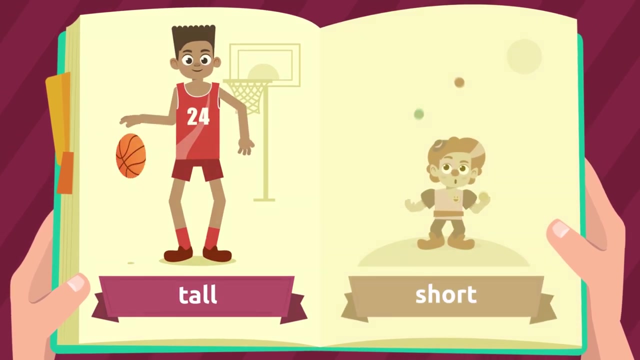 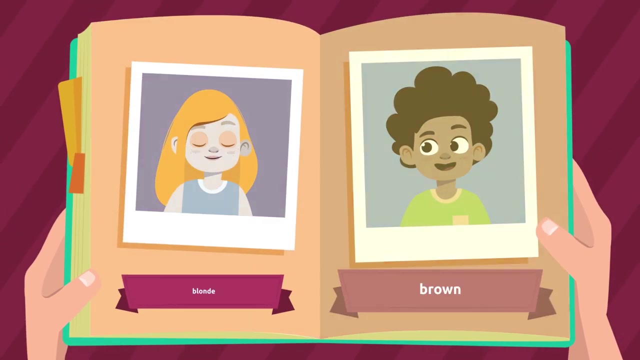 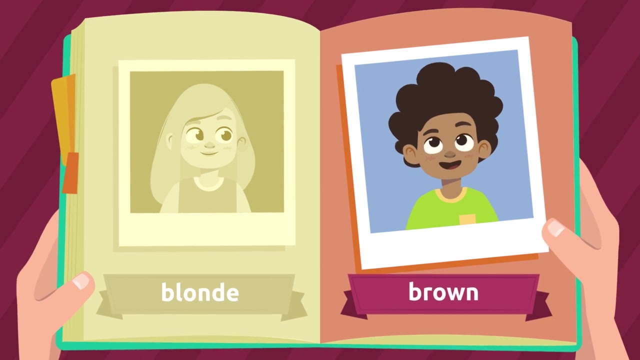 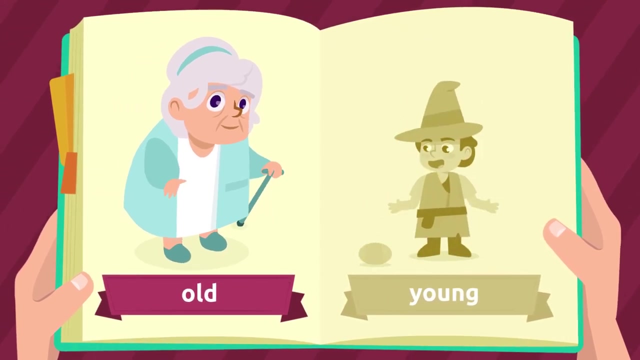 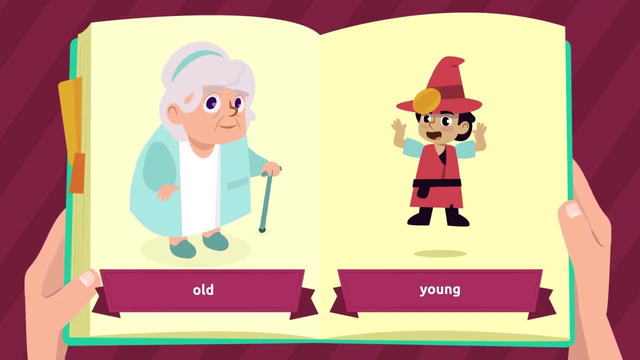 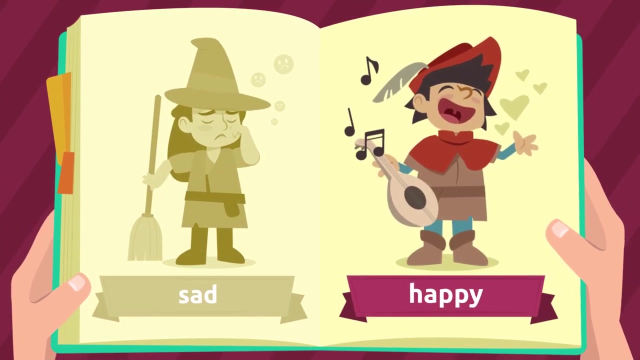 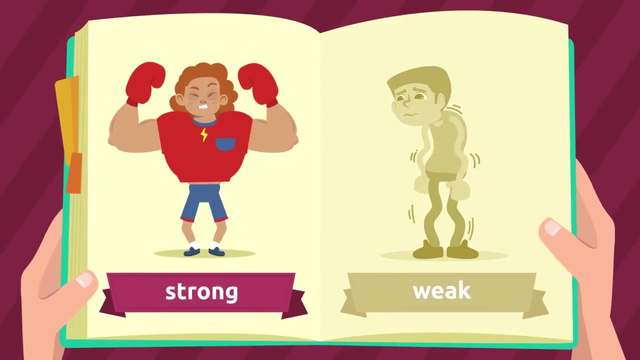 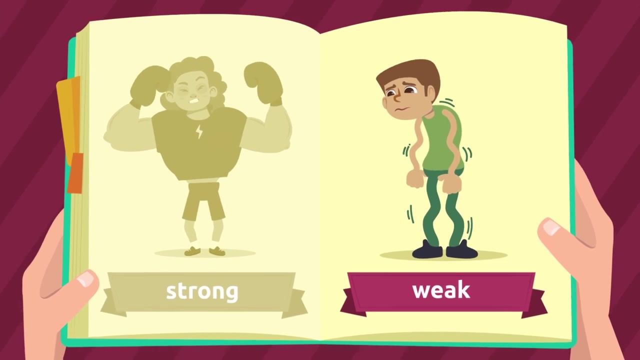 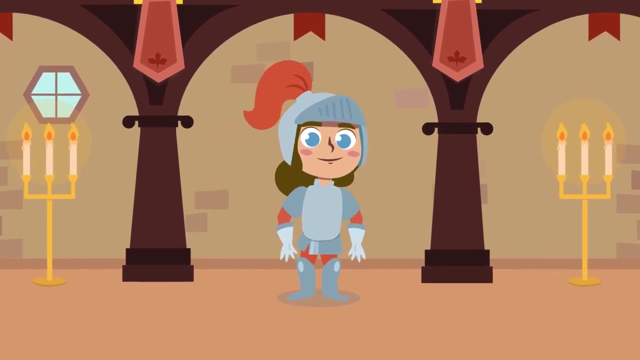 Repeat after me: weak, strong. We've learned a lot of adjectives about these friendly people. Let's review them: Tall, Short, Blonde, Brown, Old, Young, Sad, Happy, Strong, Strong, Weak, Good job Adjectives are super fun In this video. we've learned a lot about 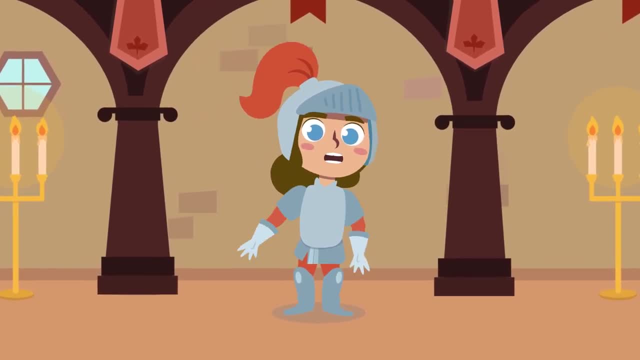 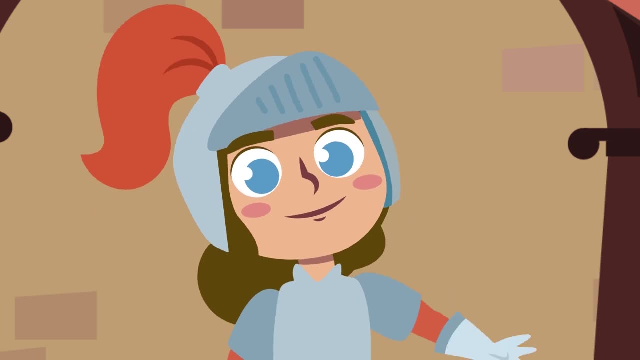 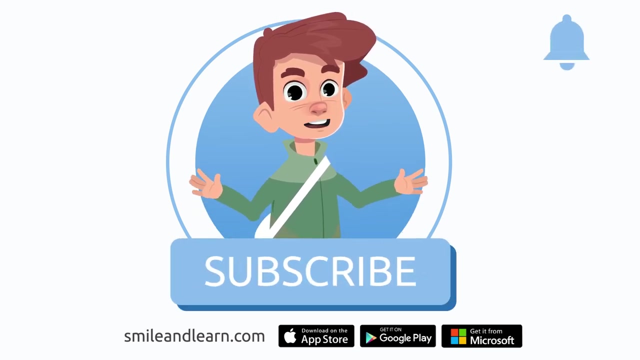 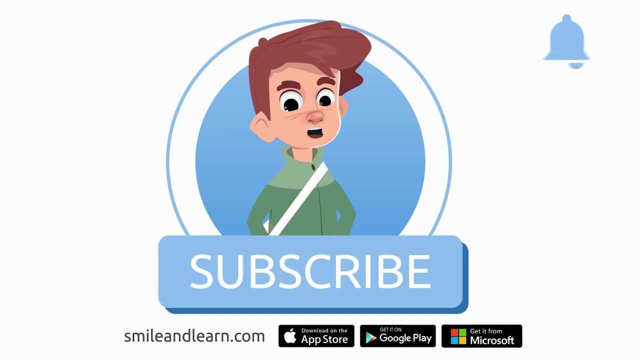 them with some people. In the next one we will learn more, but this time with places. Don't miss the next video.